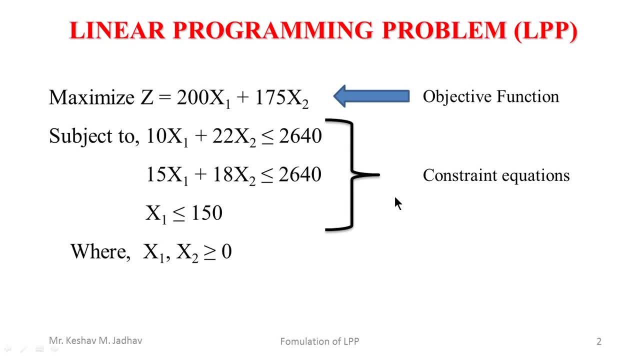 So these are the constant equations and there is non-negativity. constant x1 and x2 are greater than or equal to 0. Here we have to find out values of x1 and x2 such that the z value will be maximum and 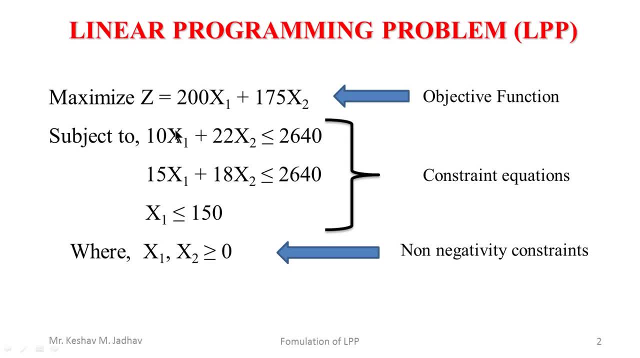 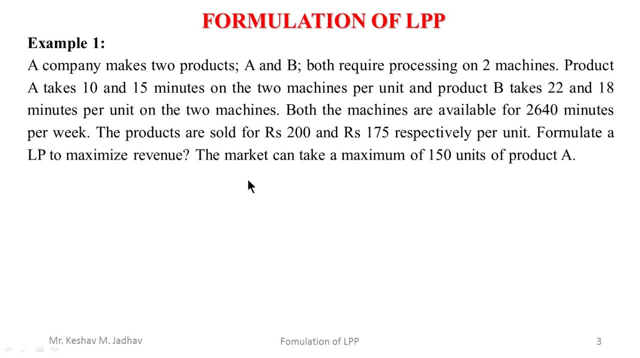 these x1 and x2 values should satisfy these constraints. So let us take an example for formulation of linear programming problem. A company makes two products, A and B. Both requires processing on two machines. Product A takes 10 and 15 minutes on two machines per unit and product B takes 22 and 18 minutes. 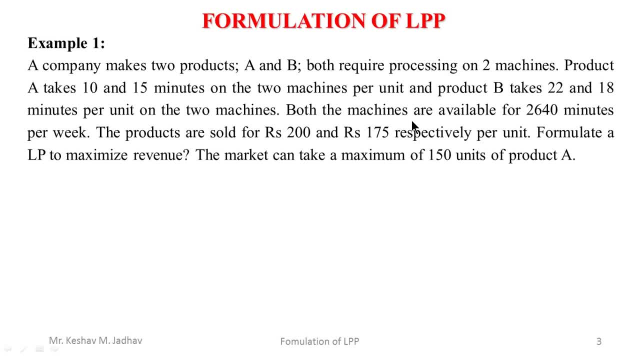 per unit on two machines. Both the machines are available for 2640 minutes per week. The products are sold for Rs 200 and Rs 175 respectively per unit. Formulate a LP to maximize revenue. The market can take a maximum 150 units of product A. 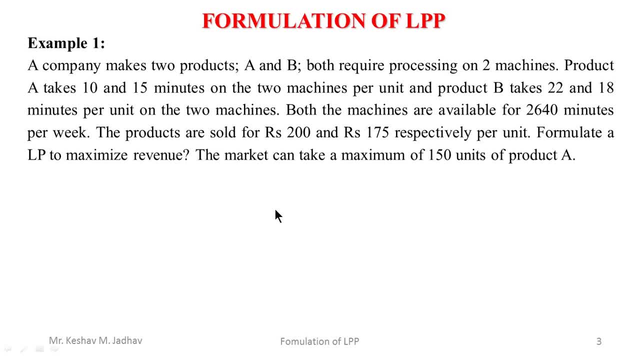 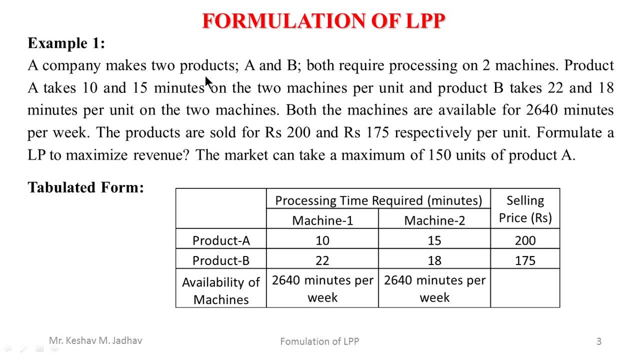 Now, first we will write this statement in tabulatory form. So here in example it is given that A company makes two products, A and B. So here we can write product A and product B. Both requires processing on two machines. So here machine 1 and machine 2 is written, And in 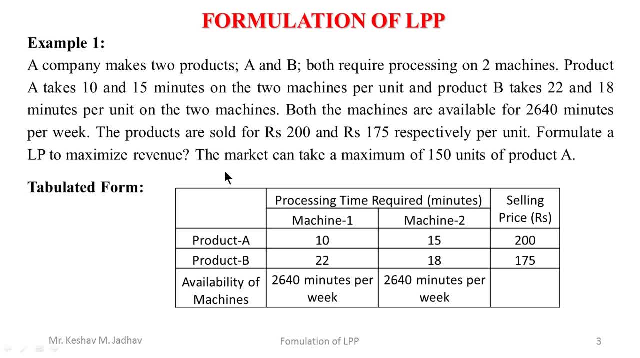 this column we will write processing time required in minutes. So here product A takes 10 and 15 minutes on the two machines per unit. So here we can write: product A will take 10 minutes per unit on machine 1 and 15 minutes on machine 2, and product b takes 22 and 18 minutes. 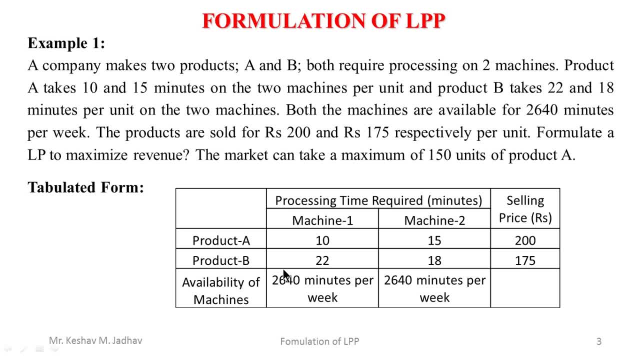 per unit on the two machines. so here we can write: product product b takes 22 minutes on machine 1 and 18 minutes on machine 2.. both the machines are available for 2640 minutes per week. so here we can add one row and here we can write the availability of the machine. machine 1 will be available. 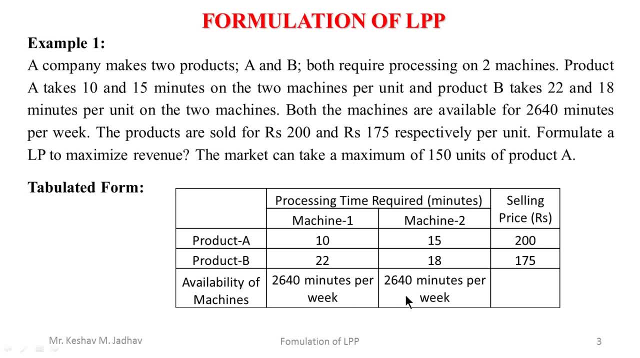 for 2640 minutes per week and machine 2 also available for 2640 minutes per week. so this is the constraint, so machine cannot be available more than this. the products are sold for rupees 200 and rupees 175 respectively, so here we can add selling price in rupees. selling price for product a is 200 rupees. 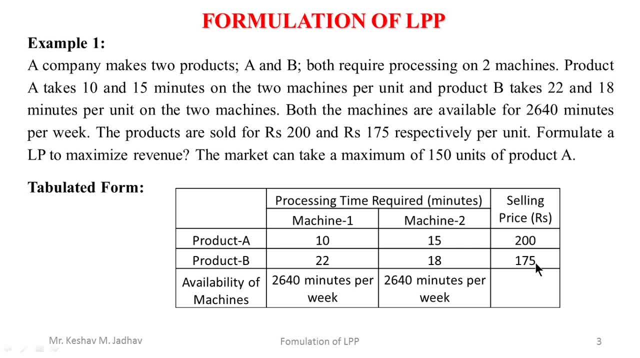 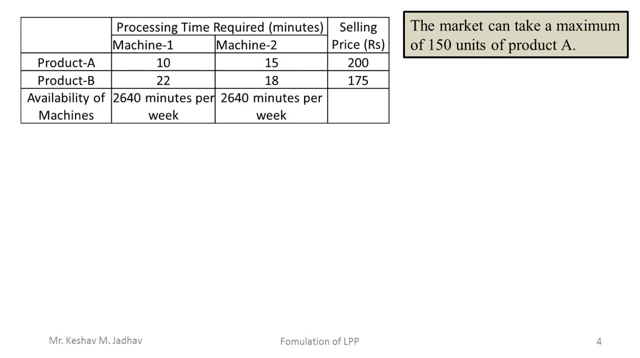 and for product b it is 175 rupees per unit. here it is mentioned that market a can take maximum 150 units of product a. after preparing this table we can go for formulation now in formulation we have to write the objective function and constraint equations for that. we have to define symbols for the variables. 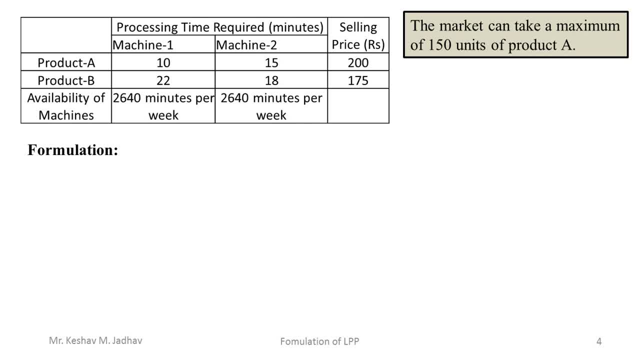 now how to decide symbols for the variables. so, to decide symbols for variable, we have to think about these two questions. first question is: what is objective? so objective is to maximize revenue. and second question is: on which parameter objective is depending. so on which parameter this is depending? revenue is depending on how many number of product a and product b we are selling. 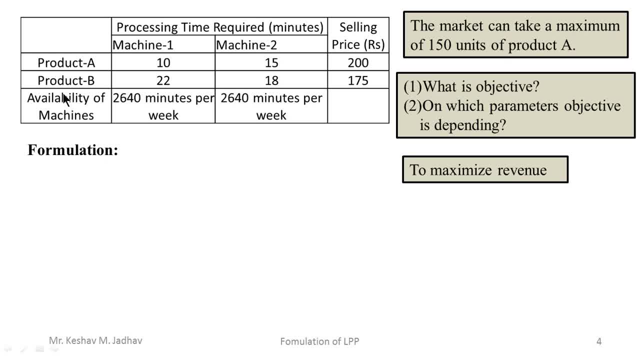 so here we have to define the symbols for number of product of type a and number of product of type b. let x1 be the number of units of product a to be made and x2 be the number of units of product b to be made. now, after deciding these symbols, 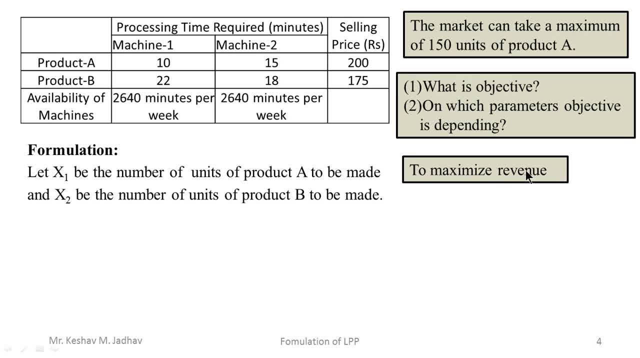 we can write the objective function. the objective is to maximize the revenue. so we can write equation for revenue: selling price of product a is 200 rupees and for product b it is 175 rupees. if we made x1 number of product of type a, then 200x1 will be. 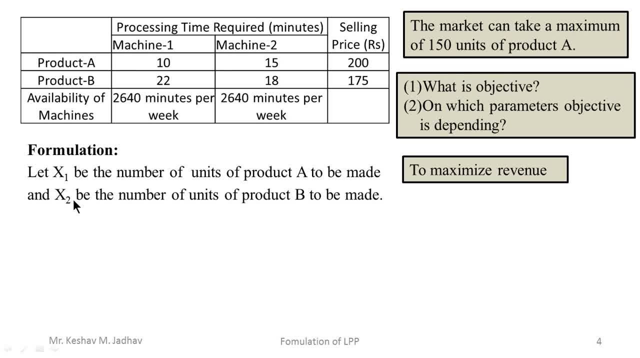 revenue from product a and if we are manufacturing x2, number of units of product b is 170 rupees product B, then 175 into x2 will be the revenue from product P. so total revenue will be: Z is equal to 200 x1 plus 175 x2. so object is to maximize this now we can. 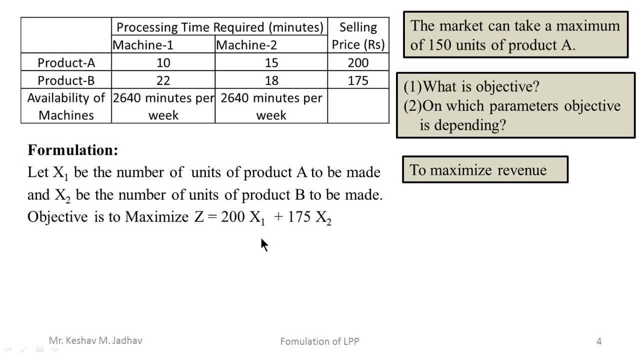 write constraint equations. now, constant it is on availability of machines, so time for which machine 1 is required, 10 into x1 plus 22 into x2, because for product A machine 1 is required for 10 minutes and for product B machine 1 is. 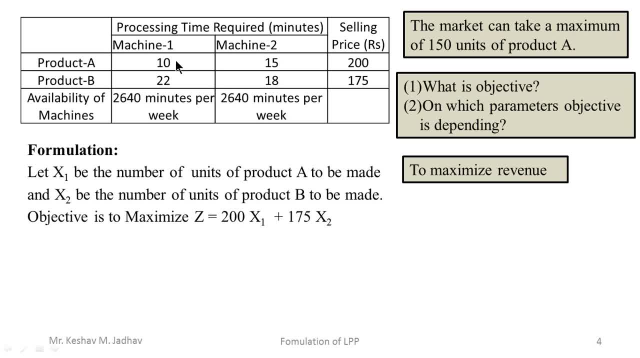 required for 22 minutes. so if you are manufacturing x1 number of product A, then 10 x1 will be the total time required for product A and 22 x2 will be the total time required for product B. so total time for which machine 1 is: 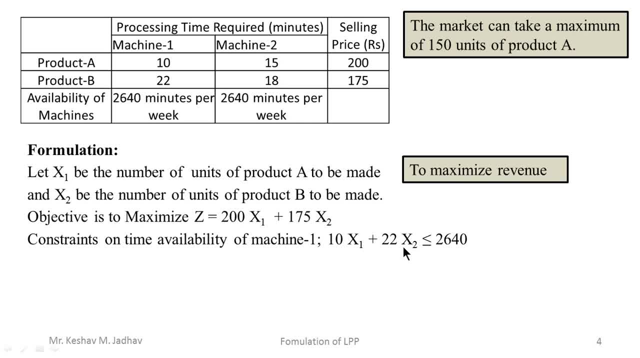 required is 10 x1 plus 22 x2, and this should be less than or equal to 2640, because machine 1 can be available maximum 2640 minutes per week. similarly, for second machine we can write: 15 x1 plus 18 x2 is less than or equal to 2640. in addition, 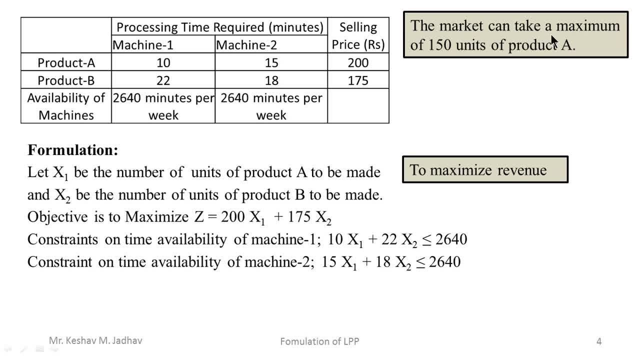 to this. in example, it is given that the market can take a maximum 150 units of product. A means x1 should not be greater than 150, so this will be the additional constant: x1 is less than or equal to 150, which is maximum quantity. 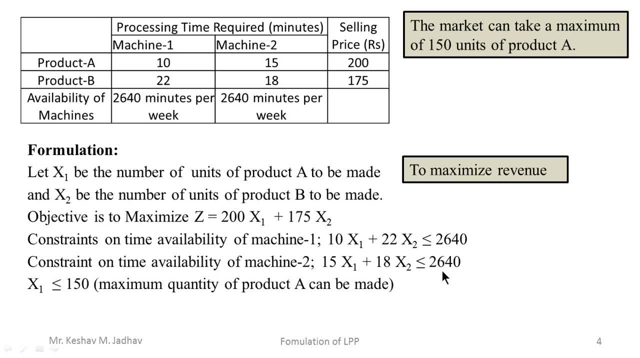 of product A can be made. so these are the constant equations. now there is no meaning for negative values of x1 and x2 means we cannot say minus one product. we can say there are two product, three product, zero product, but we cannot say minus product, we cannot manufacture minus one. 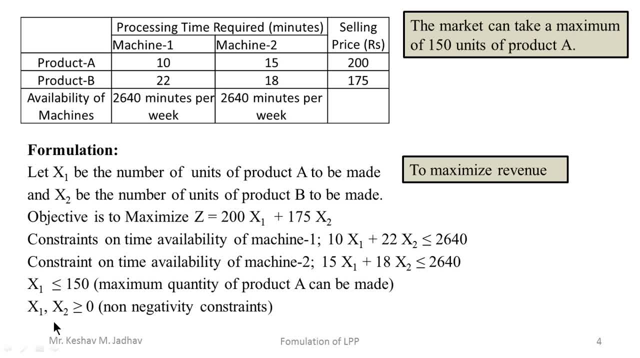 product or minus two product. so there is non negativity constant on x1 and x2. so x1 and x2 should be greater than or equal to 0. so this will be the formulation of linear programming problem. thank you.